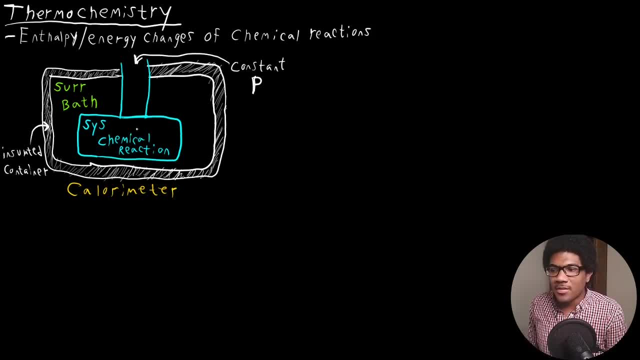 we have some sort of surrounding right. This is the exact same as our general thermodynamic system, except now we're just dealing with a chemical reaction, right? so basically, this calorimeter has some sort of outside insulated container, such that the heat transfer follows this first law of thermodynamics. 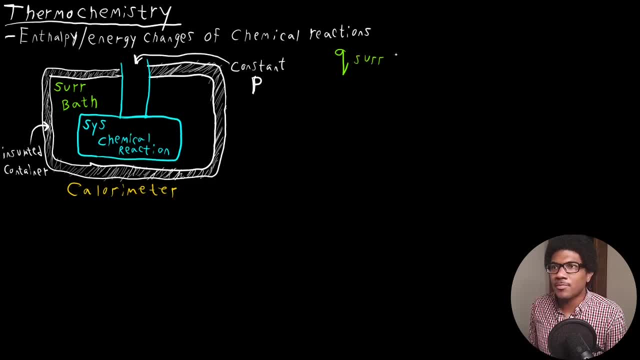 right. so where you have the Q of the surroundings plus the heat transfer of the system must be equal to zero, right? so again, that sets up that interplay where whatever heat is transferred into the system must be the negative of whatever heat is transferred from the surroundings, right? 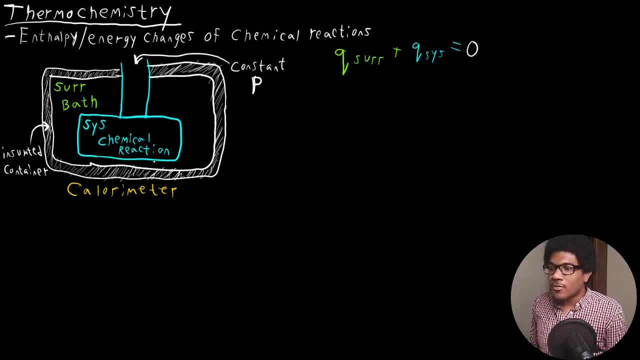 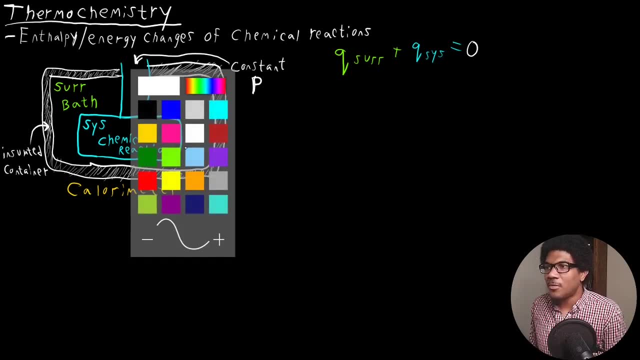 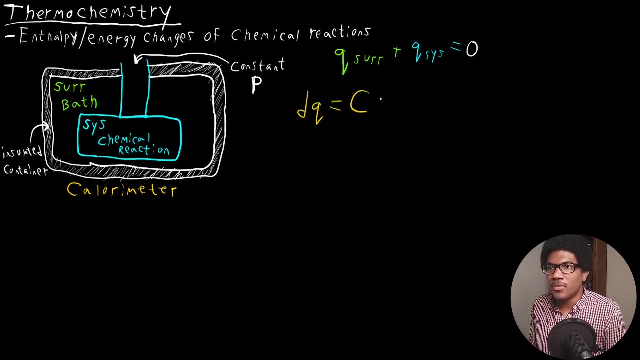 depending on the temperature, right? okay, so if we want to solve for the heat change inside our calorimeter, right, we would have to use our heat change differential equation, right? so we have: dq is going to be equal to cdt and, specifically, we're at constant pressure. so that means we're 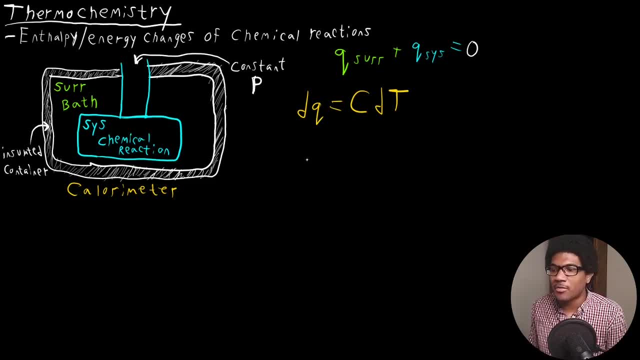 going to hold these pressures constant and be dealing with the constant pressure heat capacity. so we have dq p equals cp dt. okay, so when dealing with the calorimeter or most thermochemistry mostly, you're going to be making measurements in the bath, right? so what do I mean by that? so you're just like with the bomb calorimeter, keep in mind. 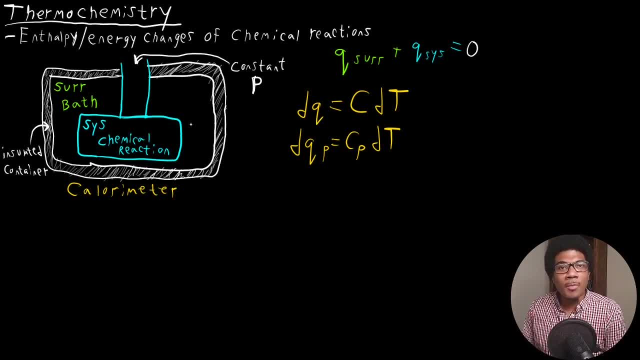 it was inside a vessel and there was no thermometer or anything being put inside the vessel or inside the reaction container. all the measurements are done outside the container or outside of the chemical reaction in the bath, right? so if we're going to add the thermometer to this, right we? 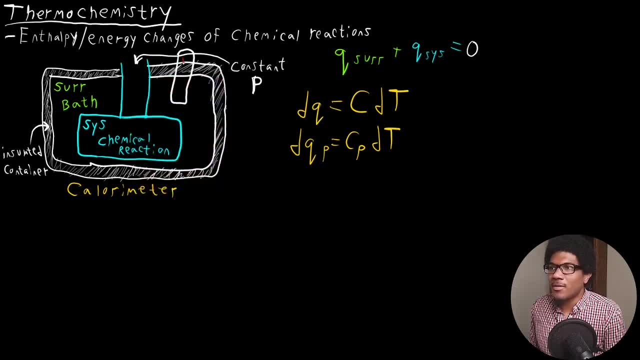 have a thermometer in this calorimeter, right, and this guy would be measuring your temperature, but it would not be in the reaction vessel, it's going to be in the bath, right. so you make all of your thermodynamic measurements in thermochemistry in the surroundings. so I'll put that: all measurements are made in the surroundings. 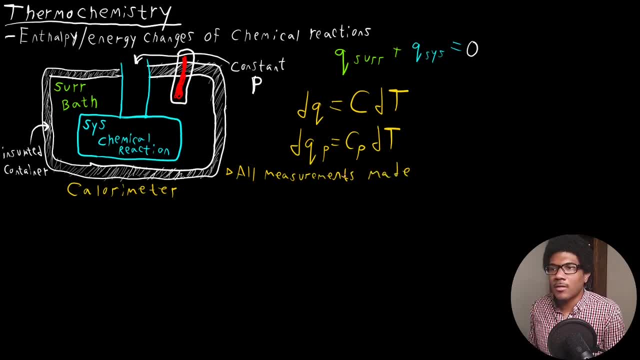 made in the surroundings, right? so, uh, basically, what we're going to have here is our uh heat change at constant pressure for the bath is going to be equal to the heat capacity, again, of the bath times. the temperature change and that temperature change you're measuring, uh, the temperature change of your bath. so that's going to be equal to the heat capacity of the bath. 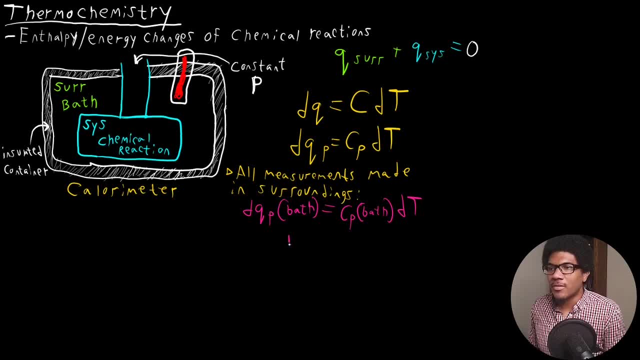 right. so since we're measuring the temperature change, let's isolate dt here, right and so if we do that, we have dq p of the bath right over the heat capacity of the bath. okay, and so we've shown that the heat capacity at constant pressure is the enthalpy right. so we can. 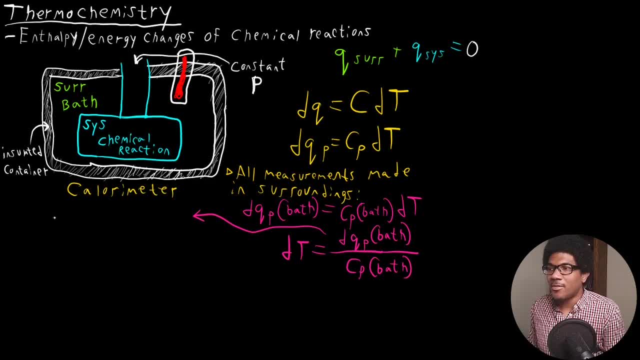 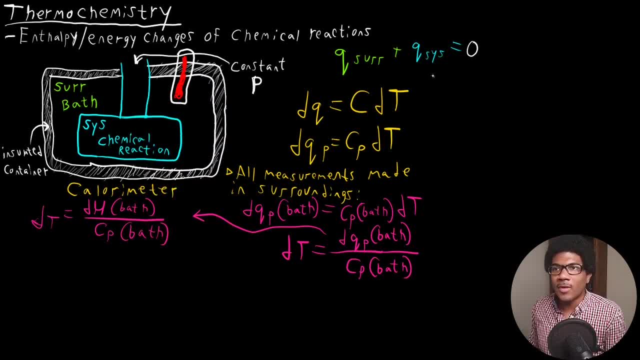 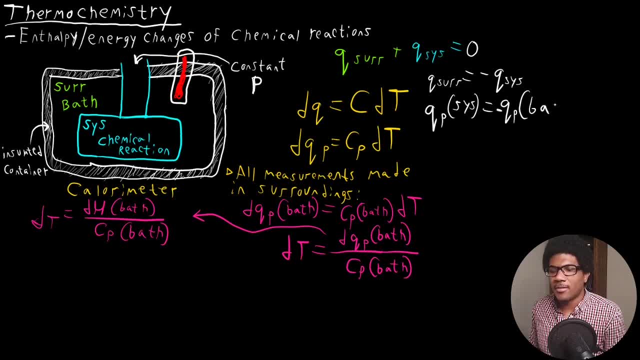 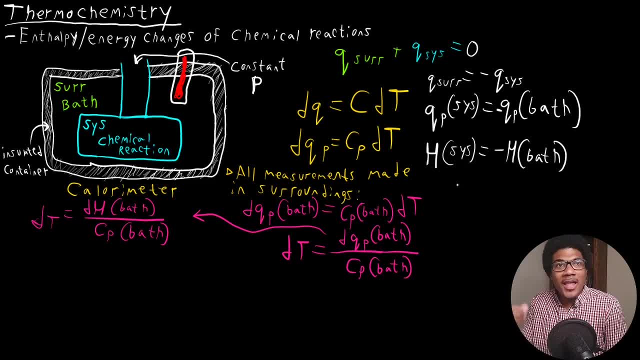 in the bath but still be getting to the enthalpy change of our chemical reaction. right since we know that all of the heat that's transferred to the bath has to be coming from the chemical reaction, we can really measure the enthalpy change of the reaction while still taking measurements. 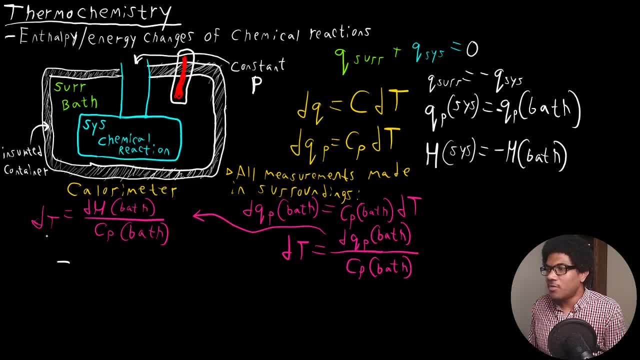 in the surroundings, right? so all we have to do is just change this equation. switch back to my little pink color there. so all we have to do is change this guy. so we have: dt is equal to negative delta h of the system over the heat capacity of the bath. 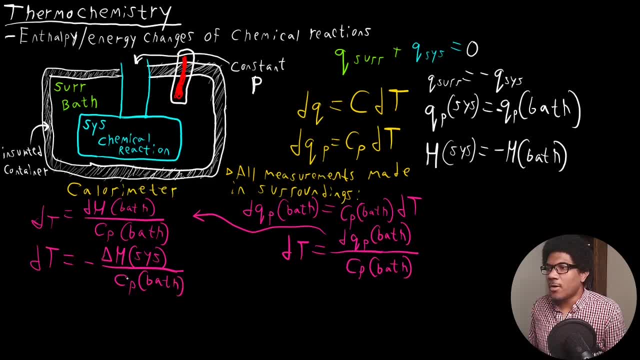 right, so? um. so think about it like this, right so? um. all we have to do is just change this guy so we have dt is equal to negative delta h of the system. all we did was just plug in, right. so if you solve this guy for h bath, that's just going to be. 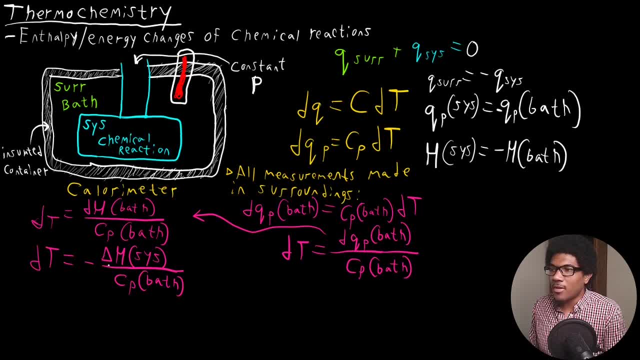 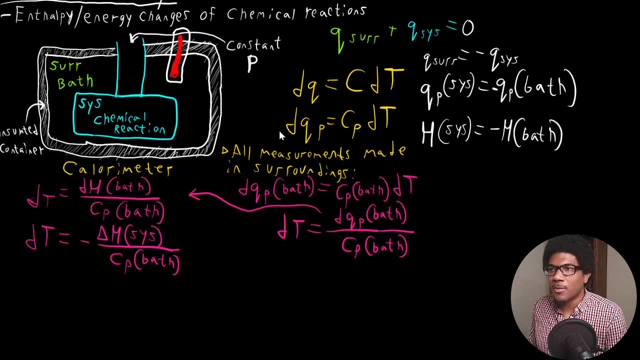 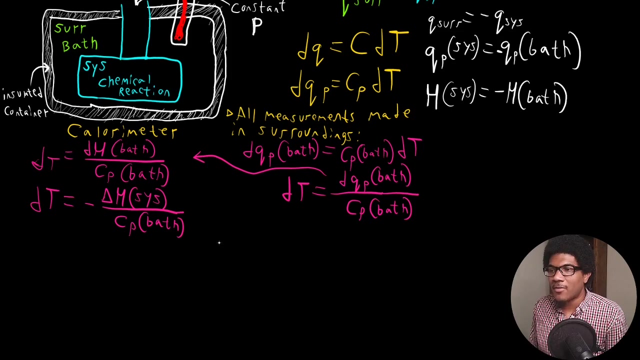 negative h system. so the same thing we just plug in here to get the temperature change right. okay, so now this gives us, um a way to define and classify, um what happens when we have an increase in temperature versus a decrease in temperature, right? so um, in this case, if we have a delta,